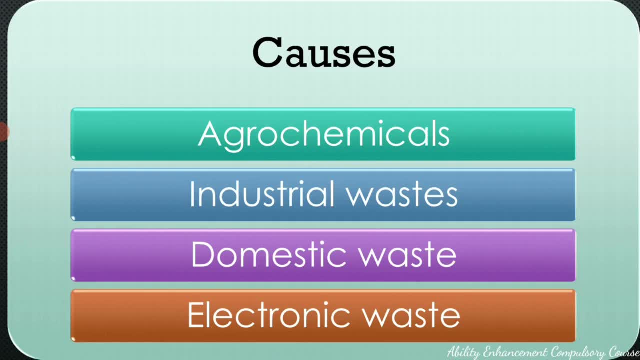 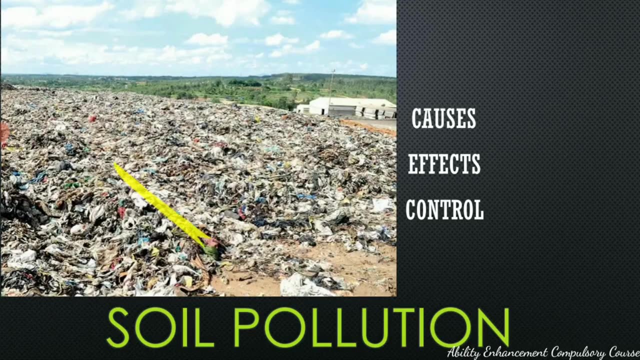 to the soil. We have even domestic wastes, for example, leakage from the septic systems or leakage from the underground tanks or pipes, or dumping of garbage, like you can see over here. sewage effluents if they are being emptied into the soil, detergents which are being emptied. 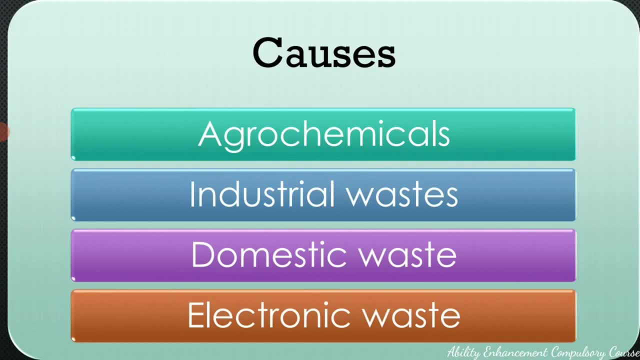 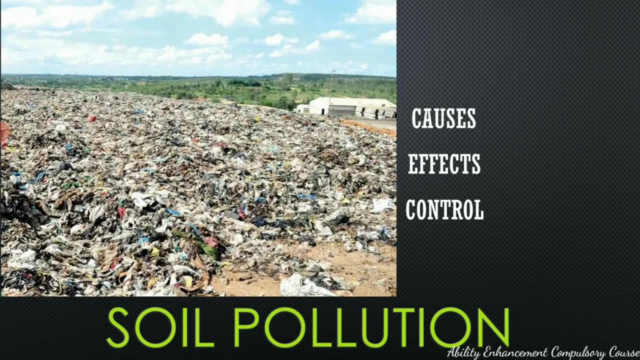 into the soil, or even you can see here in the landfills, when a large amount of waste is being stored the inside the landfill, within the garbage, there is a lot of reaction happening and there is a water coming out of it which is called as the leachate. This leachate gets into the soil. it. 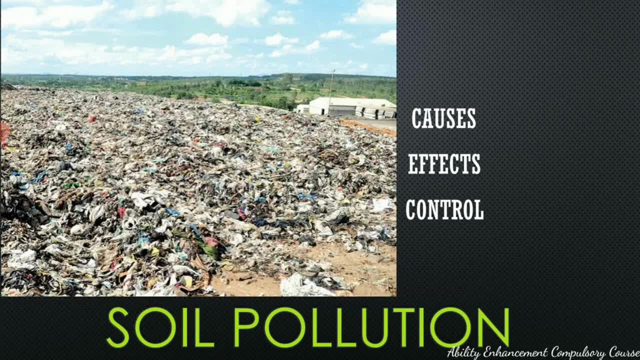 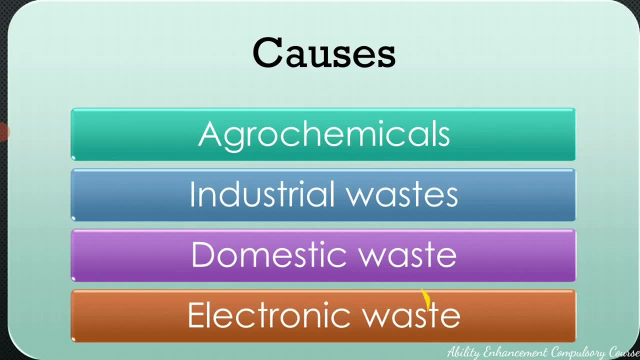 gets absorbed into the soil and then again causes soil pollution. So these are all some of the domestic wastes which are causing soil pollution. Lastly, we have electronic waste, that is, e-waste. These are the non-biodegradable substances which are having a high content of lead or cadmium, arsenic, for example our cell phones or any. 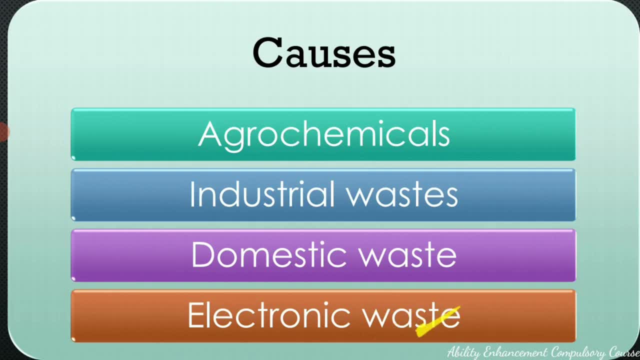 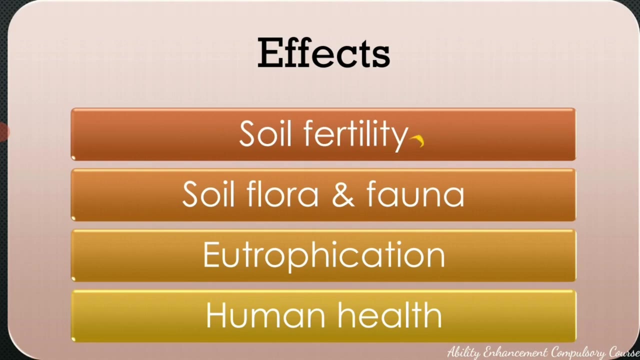 other electronic gadget that constitutes the electronic waste. So these are the different types of soil pollutants, or this is where the soil pollutants are getting in into the soil. The effects of soil pollution can be on either the soil. it can affect the soil directly, that is, it is affecting the environment in various 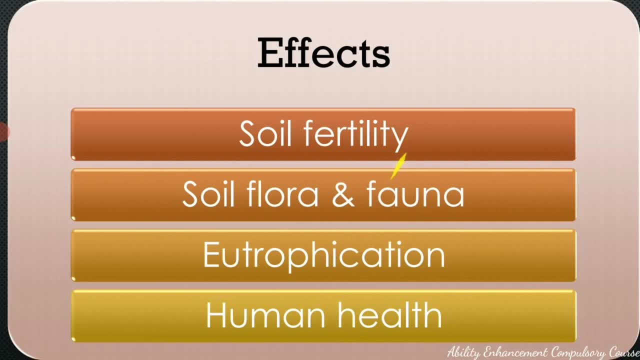 forms or it can affect the human health. When we see the soil fertility, there is definitely a loss of soil fertility, The reason being these pollutants start accumulating in the soil and they degrade the quality of the soil. So over a period of time, the plants are unable to grow over there and that 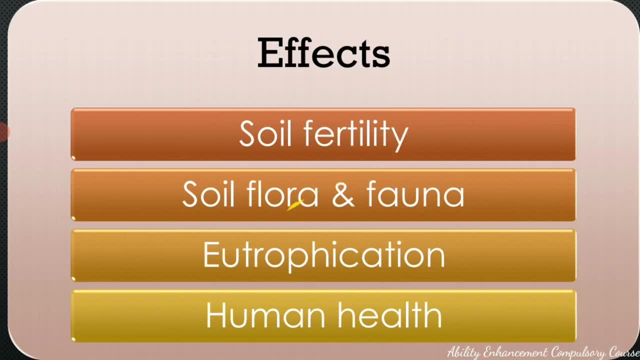 leads to a loss of soil fertility. When I say plants are unable to grow, it means even the fauna, the insects, the plant species, all of it. the biodiversity of that entire region reduces because of the presence of the soil pollutants. We also have eutrophication, which is seen in the 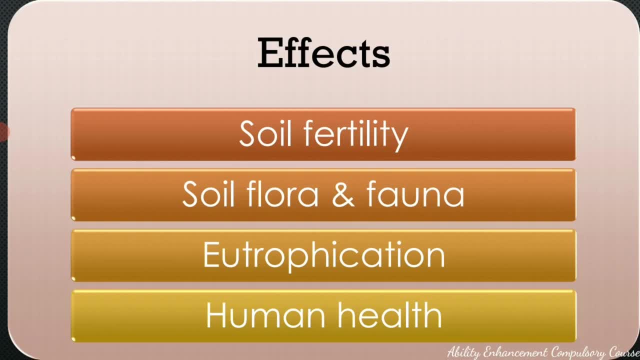 nearby aquatic bodies. We had discussed about this in our previous lecture as well. Eutrophication is when a particular water body gets enriched with nutrients, So all the nutrients which are there in the soil here may not stay within the soil. At times there could be a rain that comes. 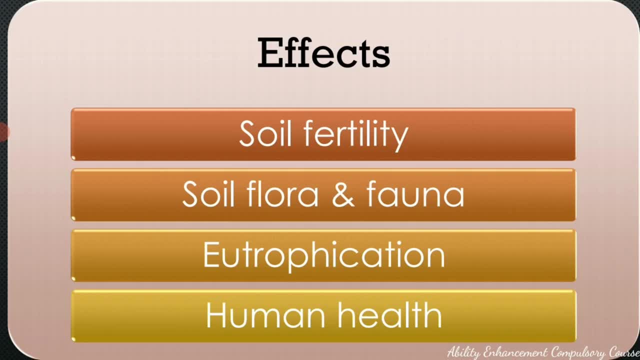 in and along with the rain, the pollutants, the nutrients from the soil enter into the aquatic body, into the lake or into a pool that is nearby. Now the problem is those aquatic bodies then retain that particular chemical and then there is algal bloom over there and you have a lot of 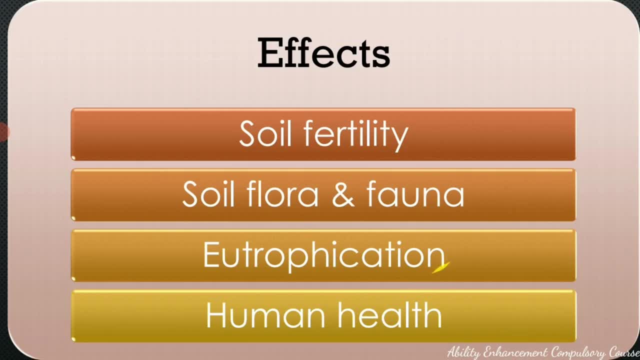 toxins that are getting deposited over there. So that is what is called as eutrophication. Eutrophication is, you can say, like a side effect of soil pollution. So not only does the soil get polluted, but even the nearby aquatic bodies take the brunt of it. 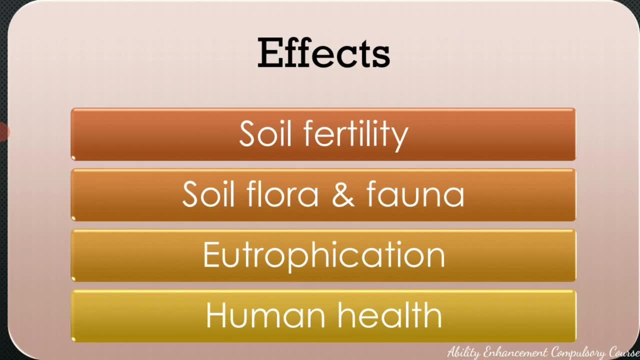 When we talk about the eutrophication, we talk about the eutrophication of the soil, When we see the human health. now, human health gets affected due to biomagnification. So this is one example wherein endosulfan, which is an insecticide, now it is being phased out globally. 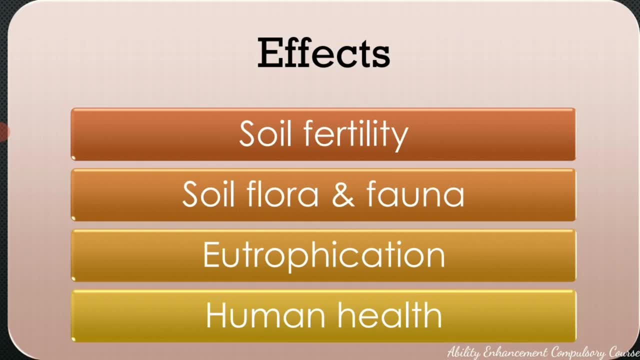 but it became a highly controversial chemical in agriculture because it was very, very effective in agriculture to kill the insects, but it was extremely toxic and, due to the phenomenon of bioaccumulation, it was causing a lot of- you know- endocrine dysfunction in the people. 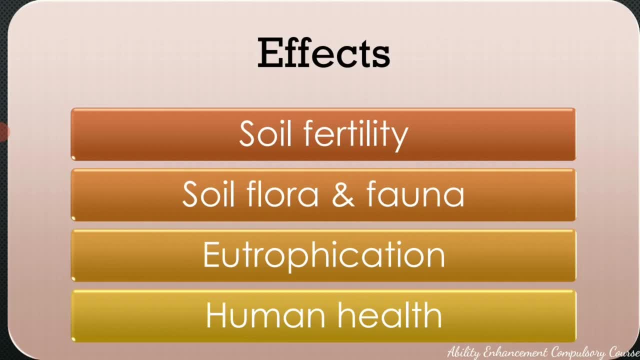 around that region. For example, in Kerala over a period of 20 years, endosulfan, which was being sprayed in the cashew estates of Kasargod district in Kerala over a period of time, people realized that it was causing severe health hazards and severe deaths were being caused. Even the people. 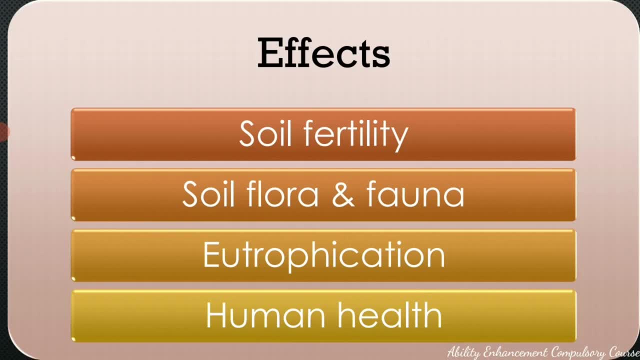 who were surviving. there was a lot of dysfunction in their endocrine system. there were mental ailments, there were physical ailments, cancer occurrences were more So. due to this, endosulfan was banned in Kerala in 2005 and then it was banned in 2005.. So this is a very big problem. 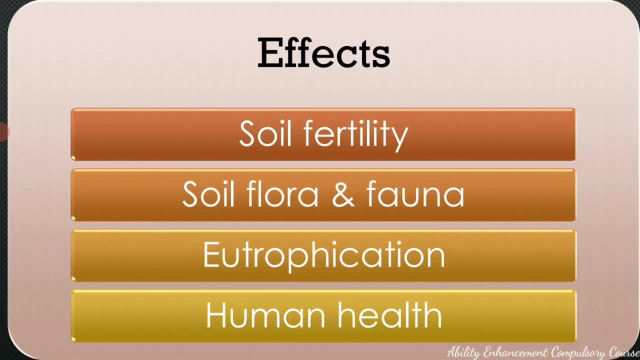 Then it was banned in India in 2011 and it is also being removed, phased out, you know, in the process of getting phased out globally. So that is one example of a chemical which may be useful in the field, but it is causing a lot of harm to the environment, to the people. 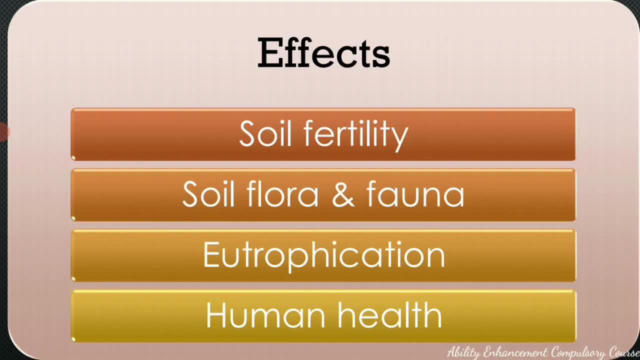 around. due to the process of bioaccumulation and biomagnification, It can also contaminate the groundwater. So when the groundwater gets contaminated and people take that groundwater for drinking purposes, then again it can affect the human health. So human health can also. 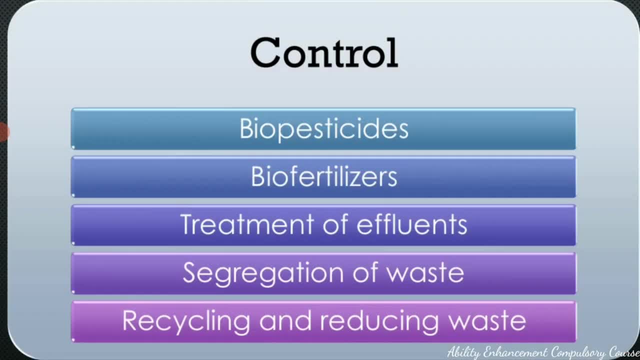 be affected, Acutely affected, by soil pollution. Coming to the control measures, the best way to control soil pollution is to shift from the chemical fertilizers, or from the agrochemicals, to organic options like biopesticides or biofertilizers. So if we go for reduction of the usage of chemicals,